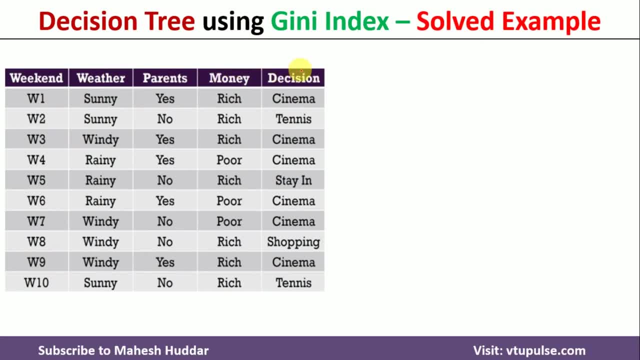 third one is money, and decision is the output variable here. The possible outputs are cinema, tennis, stay-in and shopping. There are four possible outputs are there And we have three attributes. Now, for this given data, we have to build the decision tree. 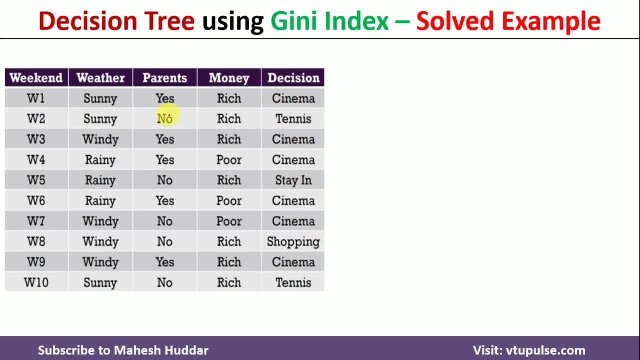 Now, if you want to build a decision tree, the very important thing we need to remember is we have to select one attribute. We need to select one attribute among the given attributes here. So in this case, we have been given three attributes, So I need to select one attribute which is having 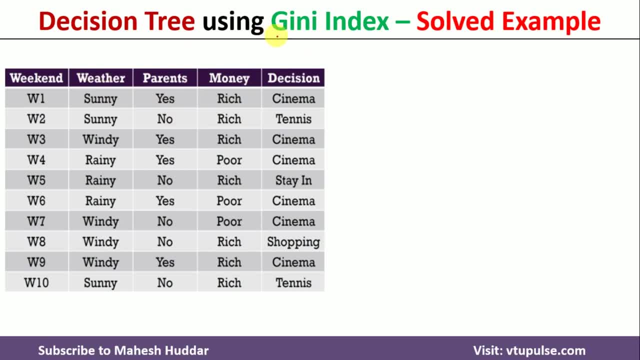 the maximum information. So in Gini index what we do is we will calculate the Gini index of every attribute. The attribute which is having the minimum Gini index is nothing, but the attribute has the maximum information. So first what we do is we will calculate the Gini of entire data set. 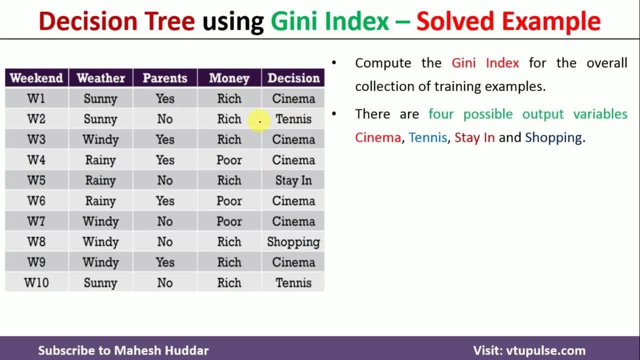 That is the whole data set you can see. So in this case we have totally ten examples. Out of ten examples, we have six instances where cinema is present- You can see here one, two, three, four, five and six- And two instances where tennis is present. So one and two where 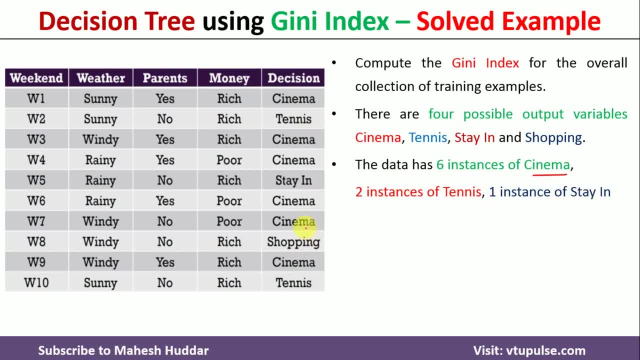 tennis is present And one instance where stay-in is present and one instance where shopping is present. So totally we have ten instances. Now for this ten instances, the Gini of total data set, that is S, is equivalent to one minus within square bracket. we have to calculate the summation. 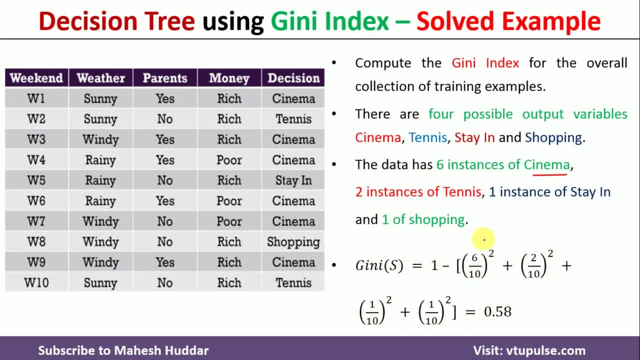 term here The summation of the proportionate instances for every possible output. So in this case we have six cinema instances, So six divided by ten bracket square, plus two tennis instances are there, So two divided by ten bracket square. So two divided by ten bracket. 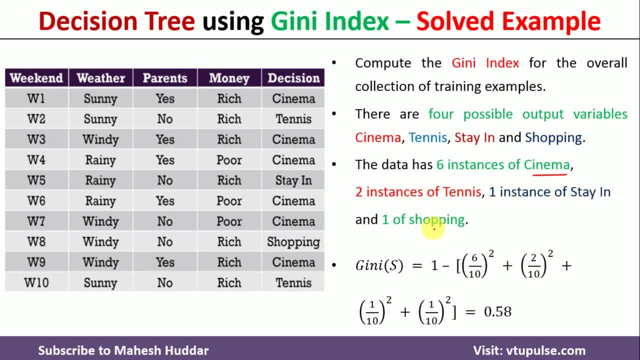 square, plus two tennis instances are there. So two divided by ten bracket square plus two tennis instances are there. One instance is of type stay-in and one is of shopping. So one divided by ten bracket square plus one divided by ten bracket square. So once I solve this equation, 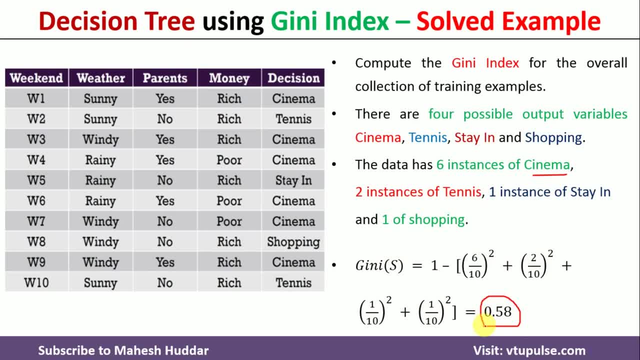 I will get Gini of this whole data set is equal to 0.58 here. So this is the process of calculating the Gini for the data set here. Now what we do is we will try to calculate the Gini for every. 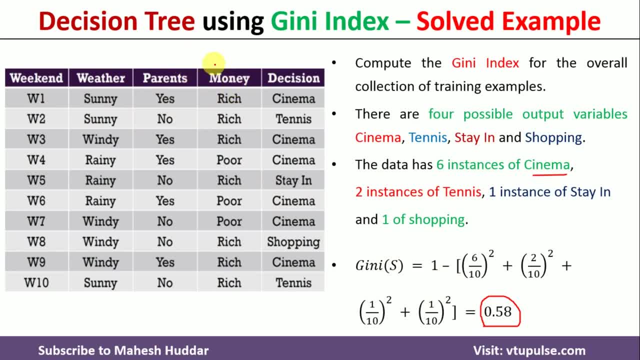 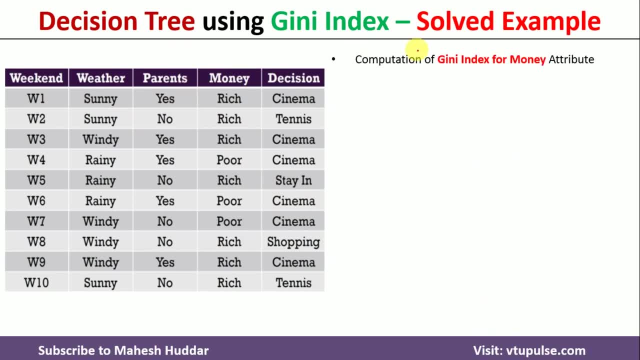 attribute and based on that particular Gini index, I will select one attribute which is as a root node, and then start constructing the tree here. So first I will try to calculate the Gini index for the money attribute. in this case The money attribute has two possibilities, As you can. 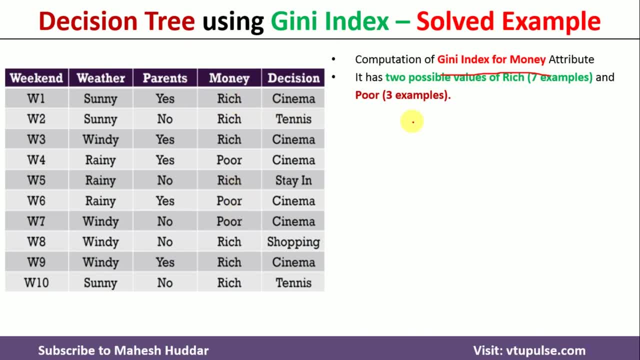 notice: one is rich, another one is poor. There are seven rich instances are there, So 1, 2,, 3,, 4,, 5, 6, 7.. There are three poor instances are there: 1,, 2 and 3.. Now, when money is equal to poor, that is. 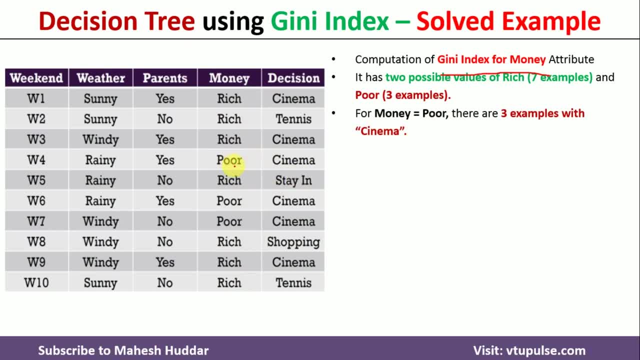 there are three instances are there, You just notice here. So poor here and the output variable is cinema, Poor cinema, poor cinema. In all three cases we have cinema as the output variable. So the Gini when money is equal to poor is equal to 1 minus the proportionate cinema. 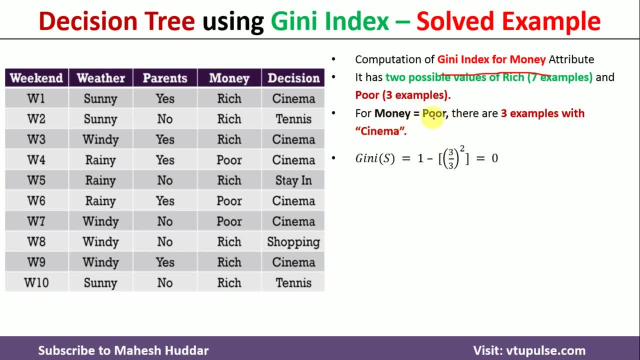 values out of the instances where money is equal to poor. So money is equal to poor is three times Out of three. all three are cinema only. So 3 divided by 3 bracket square here, which is equal to 0.. 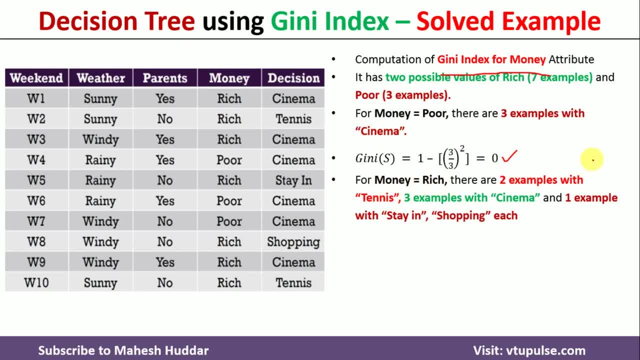 Now, coming back to money is equal to rich. So totally how many examples we have? We have totally seven examples Out of seven, two examples with the 10 is you can see here. This is the one example and this is the two examples. So two instances are of type we can. 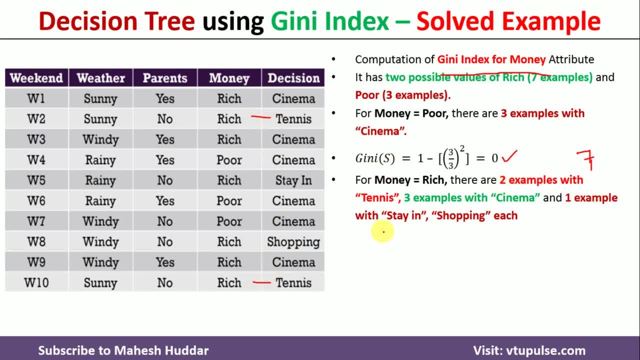 say, 10 is here and one example is staying. Three instances are cinema. That's the one more thing. So one, two somewhere it should be one more. Okay, Three instances are of type cinema, One is staying, One is shopping here. Now we try to calculate the Gini of this case, In this case, that is. 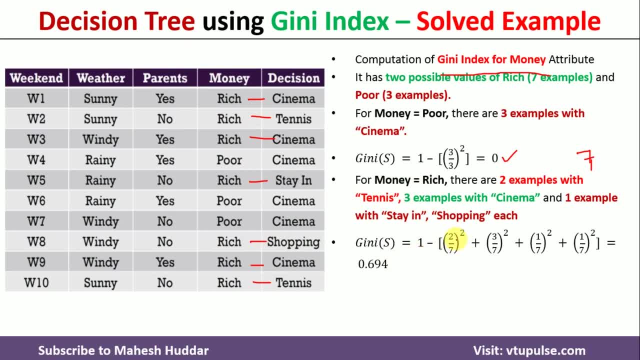 money is equal to rich, which is equal to 1 minus 2 by 7, bracket square, because the two instances of 10 is out of 7.. Three by 7, because three instances are of type cinema out of 7.. One by 7 and one by 7 because one is of type staying. 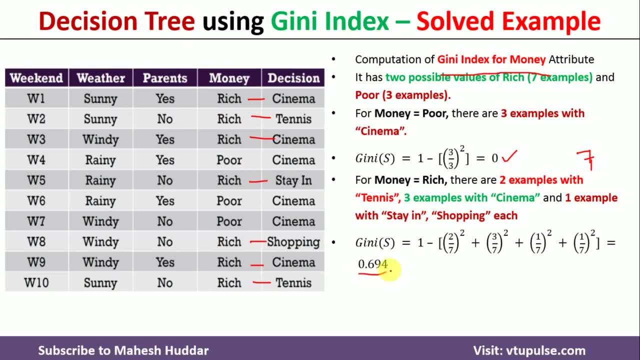 another one is also of type shopping here. So the Gini of this value is 0.694.. Now we have genie of rich as well as genie of poor. here we include these two things to calculate the weighted average for money, irrespective of poor or rich. we try to calculate the weighted average which. 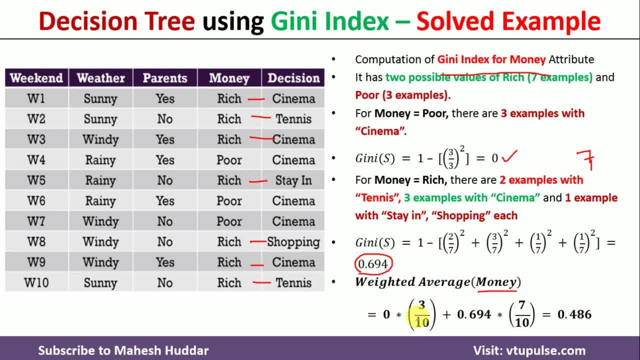 is equivalent to the genie index multiplied by the proportionate values. of money is equivalent to poor and money is equivalent to rich. so money is equivalent to poor, is three times it is present out of 10 examples. so 0 into 3 by 10 plus 0.694, that is the genie multiplied by seven times we. 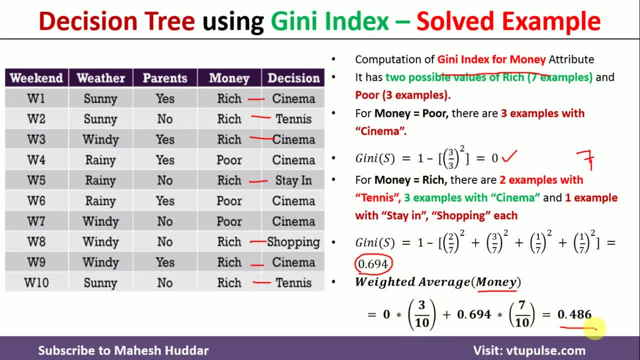 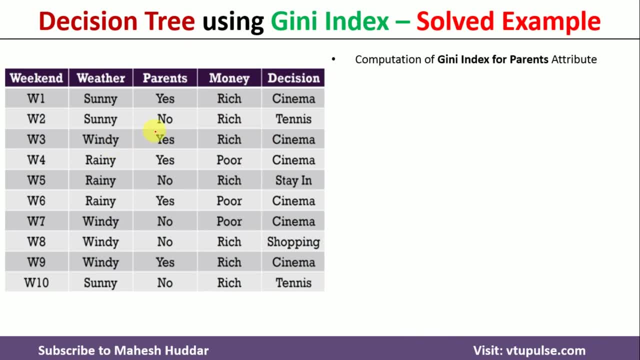 have money is equivalent to rich out of 10, so which is equivalent to 0.486 here. similarly, we try to calculate the genie for parents. the parents has two possibilities again. one is yes, another one is no. in this case, so yes, are of type 5 examples: no is of type. no is appearing five times here. 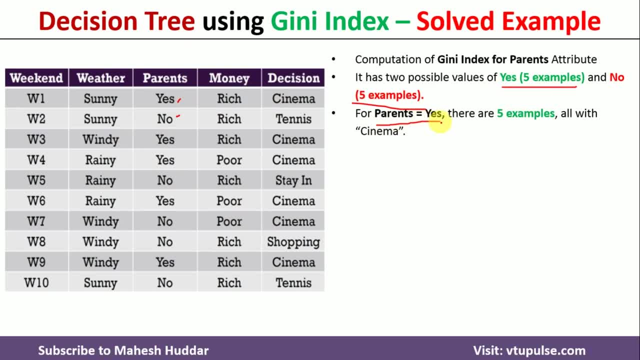 so first we consider: parents is equivalent to yes. when parents is equivalent to yes, we have five examples. all of them are cinema you can see here. so this is the first one, this is the second one, third one, fourth one and then fifth one. all of them are cinema here. so because of that, genie of parents is equivalent. 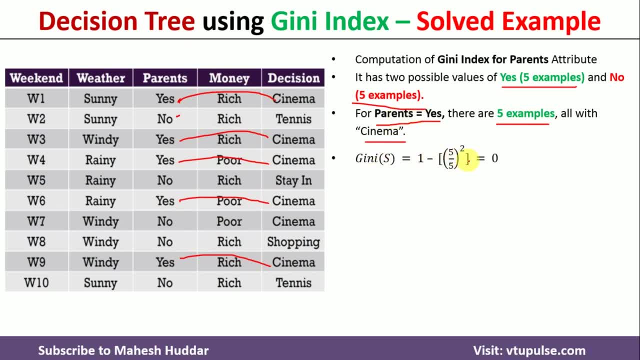 to yes is equivalent to 1 minus 5 by 5 bracket square, because we don't have any other possibilities. we have only this particular possibility when parents is equivalent to no. you can notice here: this is tennis, this is stain, cinema shopping and then tennis. the. 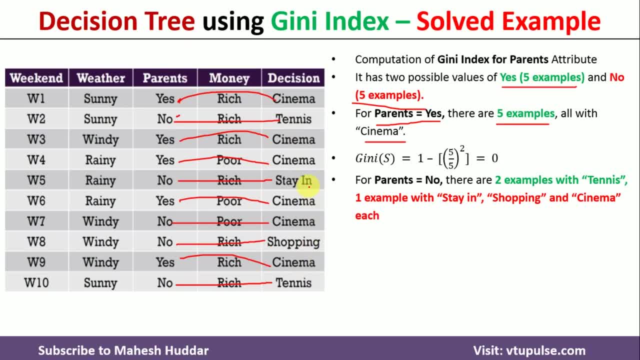 meaning is two times tennis is present, I think, one time stain is present, one time shopping is present and one time cinema is present. so totally, two times a tennis, one time stay in shopping and cinema. genie of this, that is parents, is equivalent to no, is equivalent to yes, two times fare. and the second one is a. 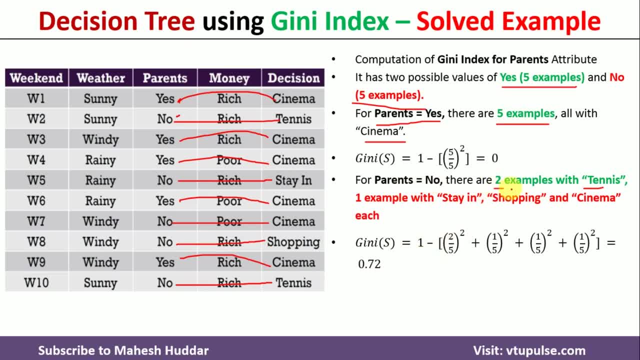 1 minus 2 out of 5, because 2 examples where 10 is present out of 5 examples remaining, all are 1: 1, so 1 by 5, 1 by 5, 1 by 5. so if you calculate this particular equation, you will get 0.72. 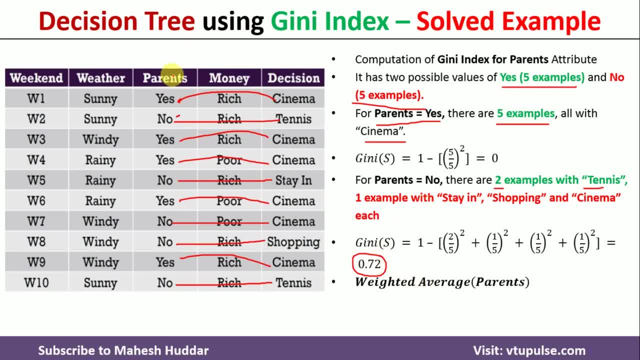 now Gini of Gini index of this particular parents is equal to 0. because Gini of parents is equal to s is 0. we have 5 examples out of 10, so 5 out of 10 here plus 0.72 is a Gini of the second one. 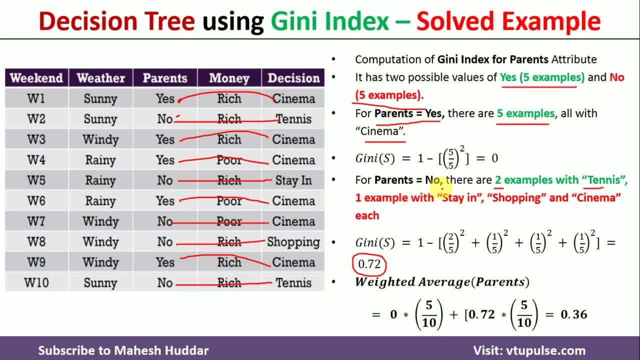 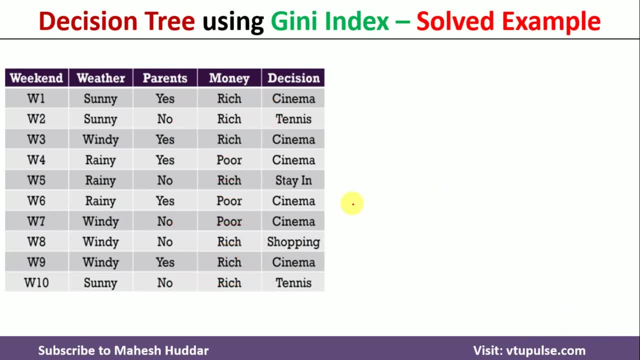 multiplied by 5. examples are there where parents is equal to 0 out of 10, so Gini index of parents is 0.36. similarly, we calculate it for weather attribute. we have three possibilities in this case: one is sunny, second one is windy and third one is rain. sunny is appearing three times. 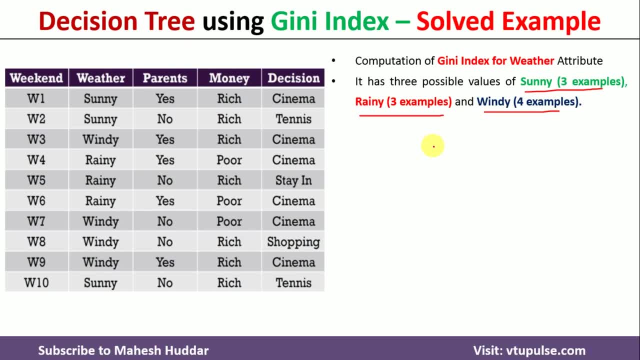 Gini of Gini is equal to 0 out of 10, so 5 out of 10 here plus 0.72 is a Gini of the second one. rain is present three times. wind is present four times. when weather is equal to sunny, we have two. 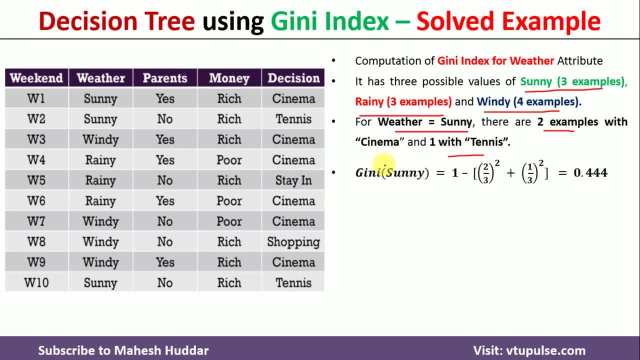 examples with cinema. one example with tennis. we calculate the Gini for sunny. similarly we calculate Gini for rain. we calculate Gini for the windy. so Gini for sunny is 0.444, Gini for rain is 0.444, Gini for windy is equal to 0.375 here. so using these three, we can: 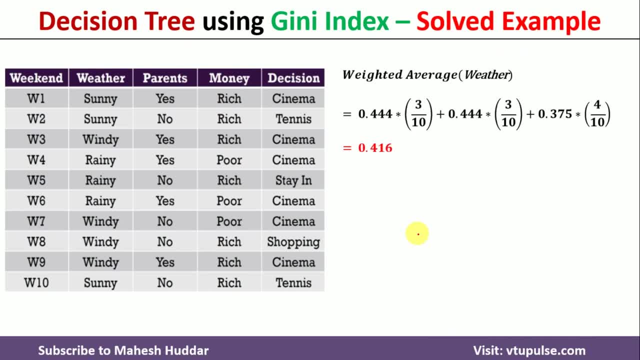 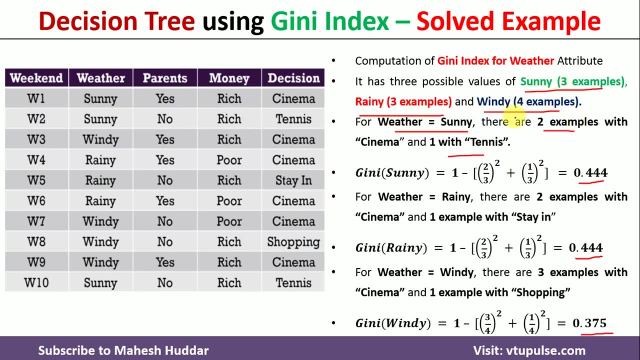 calculate the weighted. the value for a weather that is waited. average for weather is equivalent to 0.444 multiplied by 3 out of 10, 3 out of 10, 4 out of 10. so those are the number of instances opportunity here: three, three and four. so once you solve it, you will get two point four, one, six as the value here. 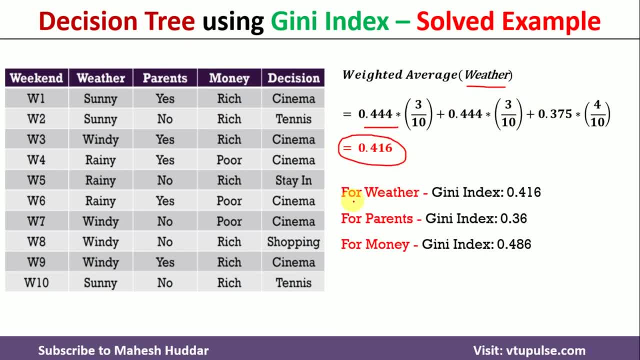 now we have calculated the genie index for all three attributes. so genie index for weather is 0.416. Gini index for payback value is less than four point four for gonna take datab, i'm going to- index for parents is 0.36. genie index for money is 0.486. year now, out of these three, the genie, 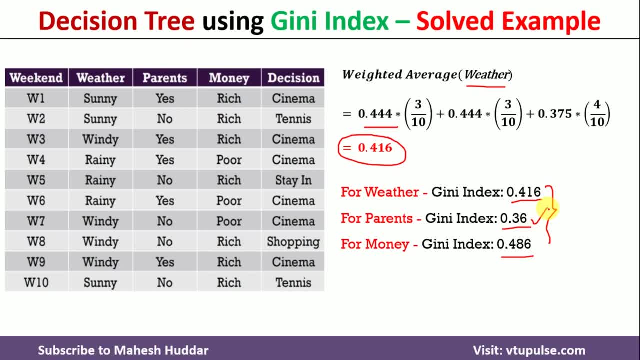 index for parents is minimum. the meaning is this is having the maximum information here. hence we calculate or select parents as the root node here. now, once you select parent as a root node, we have to divide this particular data based on the possible values of parents here. so parents has. 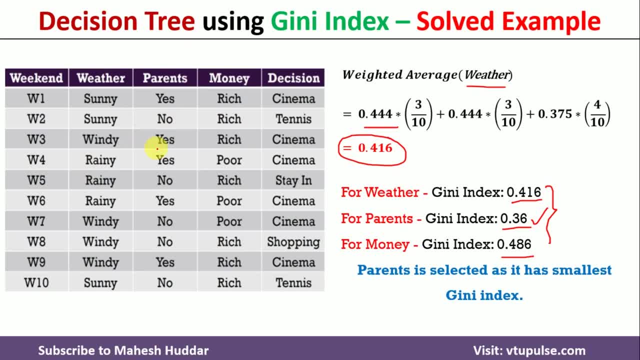 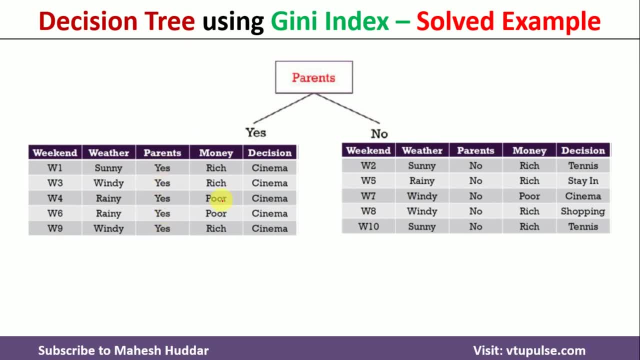 two possibilities. one is yes, another one is no. we divide this data into two parts. this is how actually it looks like. one is yes, another one is no. however parents is equivalent to yes, we will get one set of data. wherever parents is equivalent to no, we will get another set of data here. now you 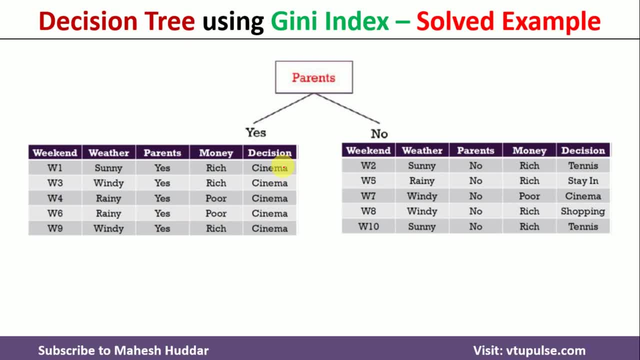 can notice, whenever parents is equivalent to yes, we have a decision as cinema all the time. the meaning of this one is: we will get the decision as cinema here. there is no need to do any computation from here onwards you. but when parents is equivalent to no, we have a combination of decisions like tennis: stay in and 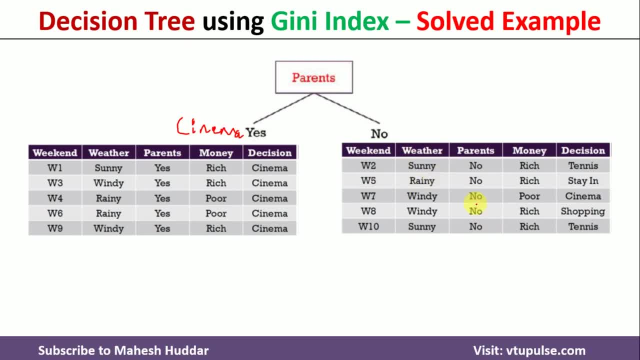 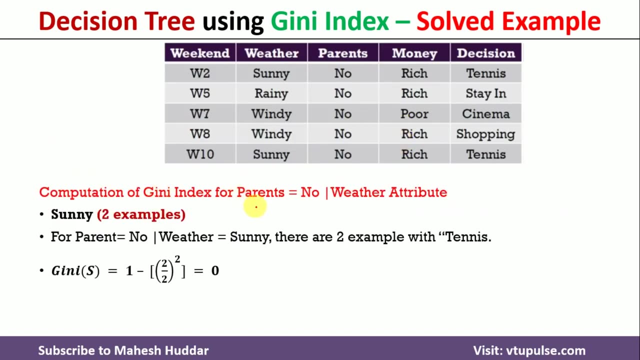 shopping. so i don't get the final answer here. so what i supposed to do is i have to use this particular subset of data and then from the remaining two attribute, that is, whether and money, i have to select one attribute over here. so that is what i did here. first i will try to calculate. 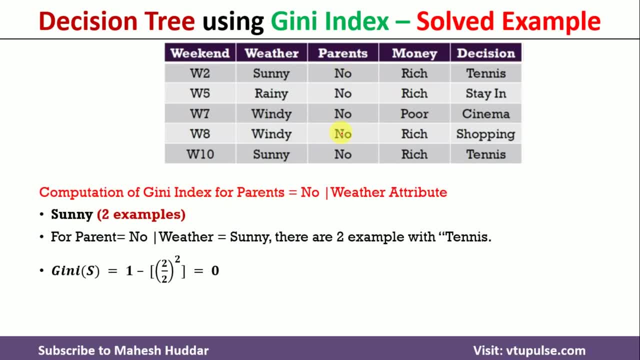 the genie index for parents is equivalent to no, and whether is the attribute so when weather is present? we have three possibilities. one is sunny. we have two examples. both the examples are of type tennis, in this case sunny, sunny tennis, tennis here. so the genie of this one is zero. and then second one is rainy. rainy is appearing one time, so one out of one, which is 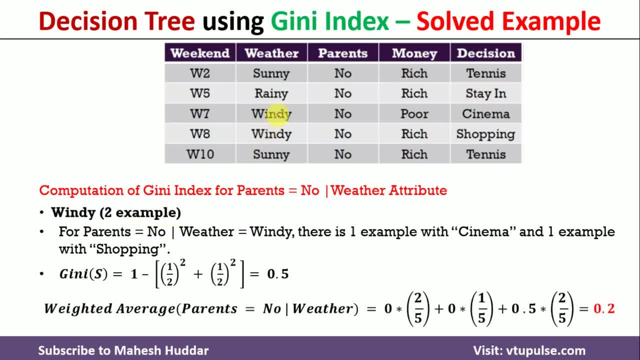 equivalent to zero again. third one is windy, so windy is appearing two times, but one time it is cinema, another time it is shopping here. so the genie of this value is zero. and then second one is: is 0.5? weighted average of parents is equivalent to no and weather attribute is equivalent to zero. 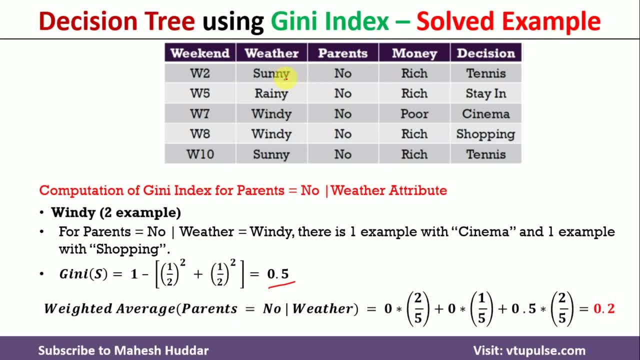 because the sun is genie is zero and it is appearing two times out of five, plus zero because the genie of rain is zero. we have already calculated: it is appearing one times out of five. the genie of windy is 0.5 multiplied by 2 out of 5, because it is appearing 2 times here. so the genie 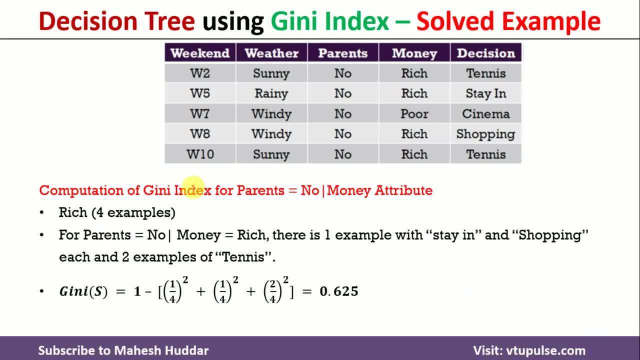 of this weather attribute is 0.2 in this case. now we try to calculate the genie index for the money attribute. it has four rich examples and two four examples out of four rich examples. one example is of type stain and another another one is of type rich here and the remaining two are: tennis in this case. so one minus 4, 1 by 4 plus 1 by 4, uh squares plus two by four bracket square, which is equivalent to 10 square, which is equivalent to 4 bracket square, which is equivalent to 2.9 by 4 bracket square. 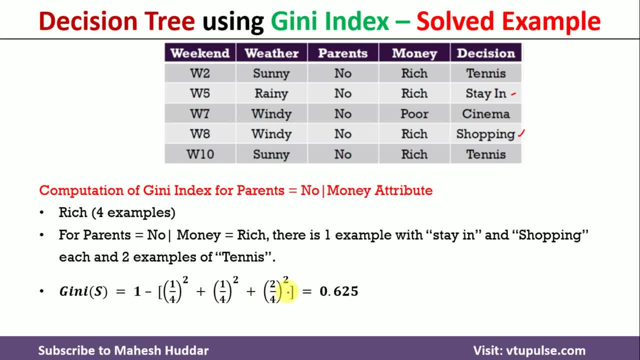 4 by 4 plus 1 by 4 bracket square, which is equivalent to 5. polar rigidity variation: 0.625. the another one is the poor, which is of type cinema: 1 minus 1 by 1 bracket square, which is equivalent to 0. here now, by considering these two things, i will get the weighted average for. 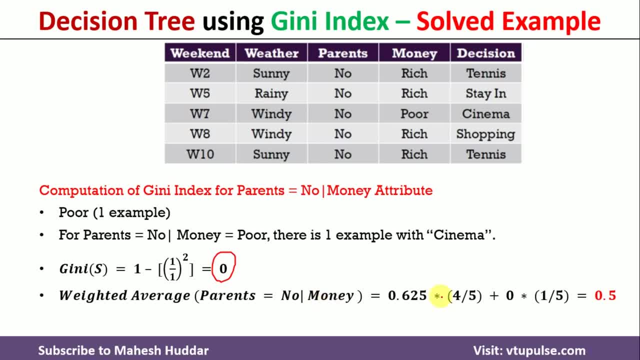 parents is equivalent to no, and money, which is equivalent to 0.625. that is the genie for rich. rich is appearing four times out of five examples plus 0 is the genie for poor, and it is appearing one out of five times, which is equivalent to 0.5. here now, the genie index of parents is equivalent. 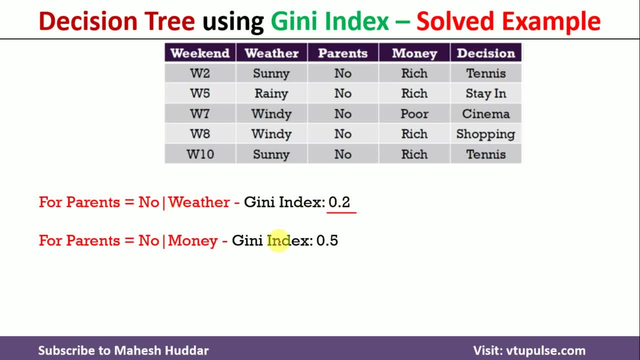 to no, and attribute is weather, which is equivalent to 0.2. genie index for parents is equivalent to no, and attribute is money, which is equivalent to 0.5. between these two, weather is the smallest one. so i will consider weather as the attribute for building the tree here. now, once i select, 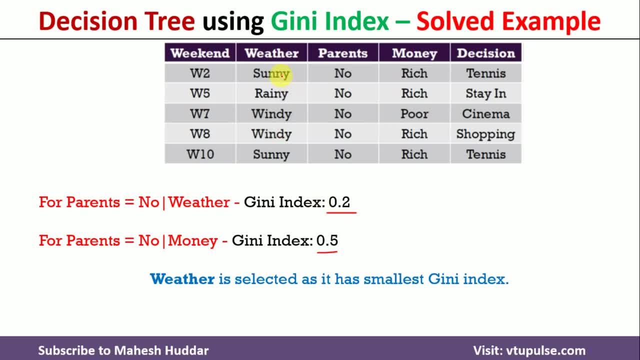 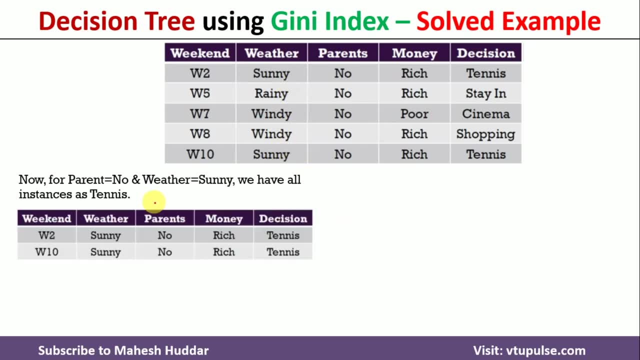 weather we have three possibilities: one is sunny, one is wind and one more is rain. so three branches we will get. so for sunny we will get the subset of data, something like this: so whenever we have sunny- that is, parents is equivalent to no and weather is equivalent to sunny- the decision is tree 10 is here, so there is no question of 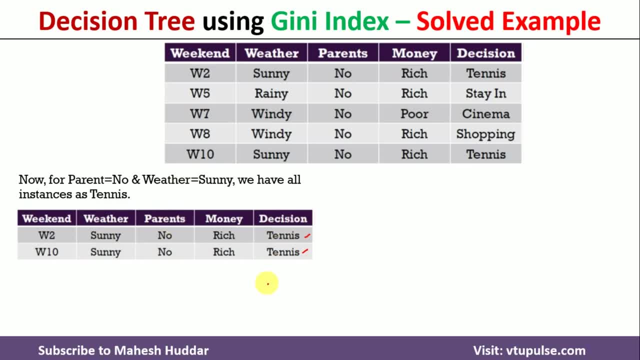 finding the best attribute. from here onwards, the decision is already: 10 is here whenever. parents is equivalent to no and weather is equivalent to rainy. that's why it is possible to get the best attribute. there is only one example and it is stain. so the answer is: stain here when it comes. 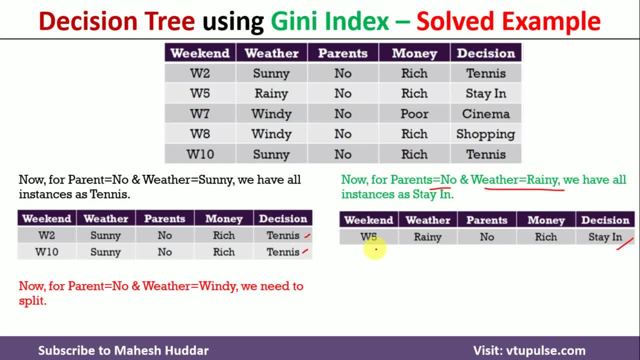 to third one, that is, when parent is equivalent to no and weather is equivalent to windy. we have two possibilities: one is the cinema, another one is shopping. so we cannot make a decision here. so what we do is we have to consider the remaining attributes. parents and weather is already considered. 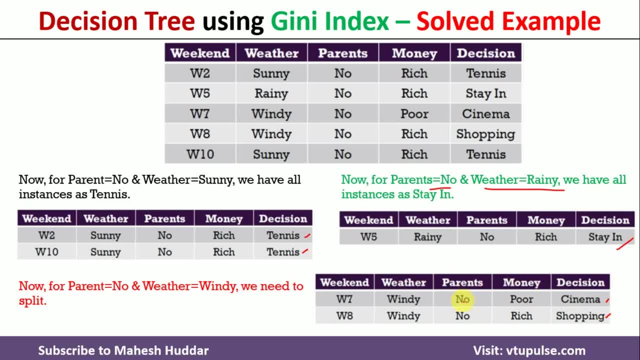 the remaining attribute is money. so when parents is equivalent to no, weather is equivalent to windy and money is equivalent to poor, the answer is cinema. when parents is equivalent to no, weather is equivalent to windy and money is equivalent to rich, the answer is shopping here. so that is how we can.